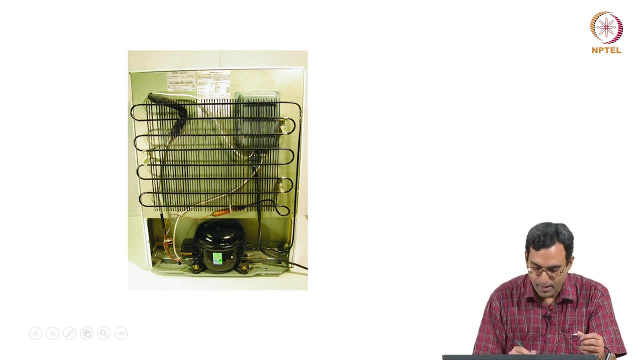 which you want to cool inside the refrigerator, And then, finally, it comes back And goes into this compressor, where it is once again compressed. So if we were to look at this on a sort of a schematic, what we see is we have components of this kind, We 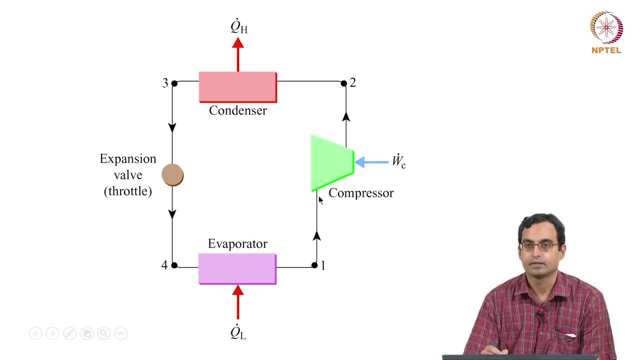 have a compressor where we take in refrigerant. we compress it. it becomes high pressure refrigerant. The temperature increases while we compress. Ideally we would like to compress this isentropically, reversibly and adiabatically, And then we compress it. 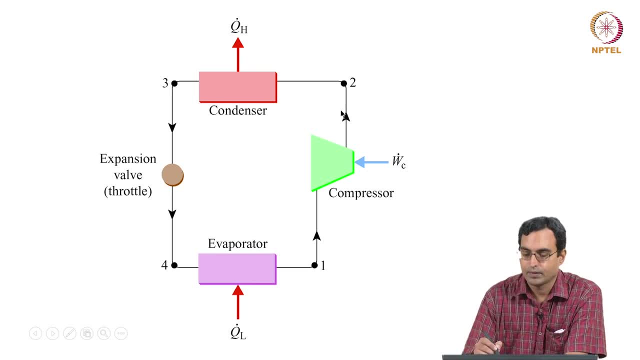 And then we compress it And after compressing we are left with high pressure refrigerant. This refrigerant then goes into a condenser where we allow it to reject latent heat and become a liquid. So it is still at high pressure, It rejects heat, becomes a liquid. This liquid is something. 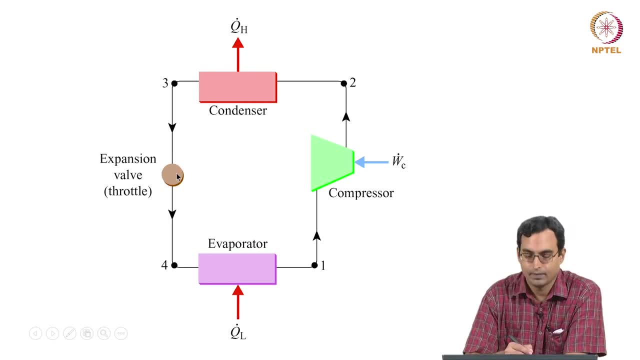 which we usually send through an expansion valve or a throttle valve. In this process, the pressure of the refrigerant reduces. This refrigerant is liquid when it enters this expansion valve. It is not an ideal gas in any by any means, As its pressure. 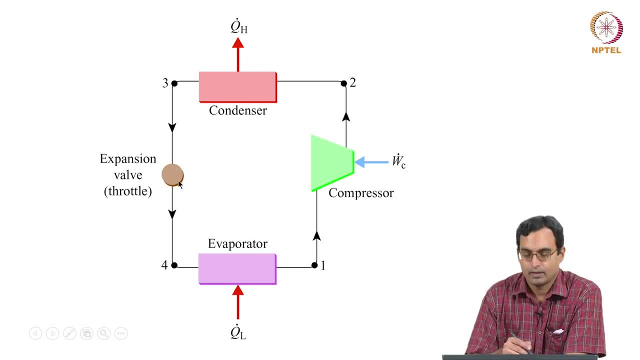 drops in the expansion valve. what we see is that its temperature drops, its quality increases, it starts to become vapor, And then we are left over here with a mixture of liquid and vapor which we send through the evaporator. This mixture is cold In the 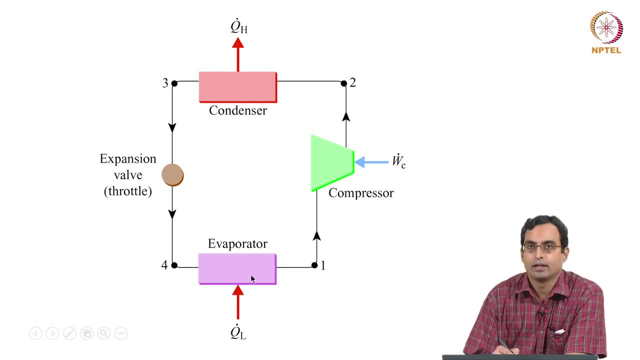 evaporator. it takes heat from whatever we have sent through the evaporator. This mixture: it is cold. It takes heat from whatever we have sent through the evaporator, And then a substance you want to cool, and then you are left with, hopefully saturated paper, which 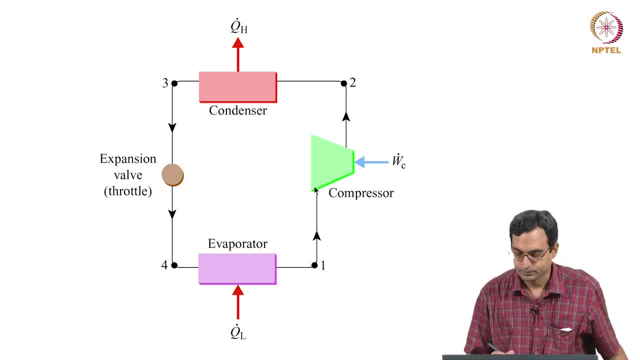 then you can send into this compressor. So this is essentially how this works. So we have work input given in the compressor, we have heat transferred out in the condenser, we have heat transferred in into the evaporator and then we have the expansion valve, which 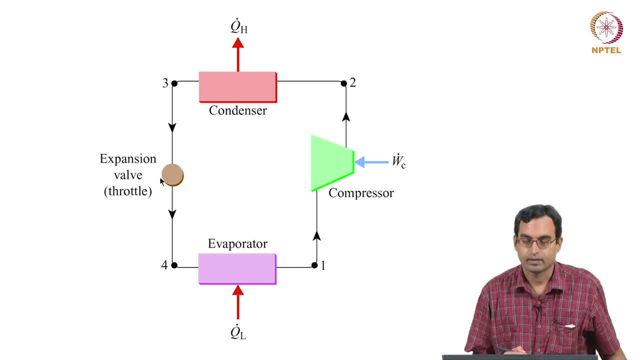 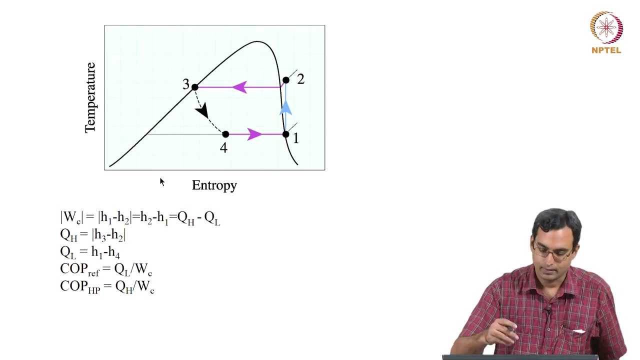 is a throttling process. We have discussed earlier that the throttling process ideally would be adiabatic. it is highly irreversible. there is no work done in this case. So we can look at this process on a TS diagram. But what we can also do is see why we use this process at all or the cycle at all. 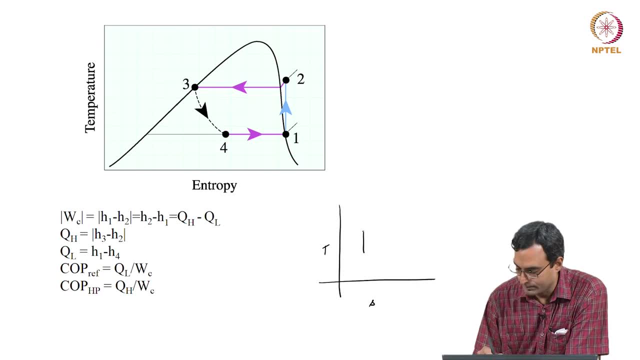 So if we were to look at Our ideal refrigeration system, the ideal refrigeration system would be a Carnot cycle running in reverse. So which? by running in reverse, what we mean is that heat is transferred out of the cycle at high temperature and heat is transferred into the cycle at low temperature. 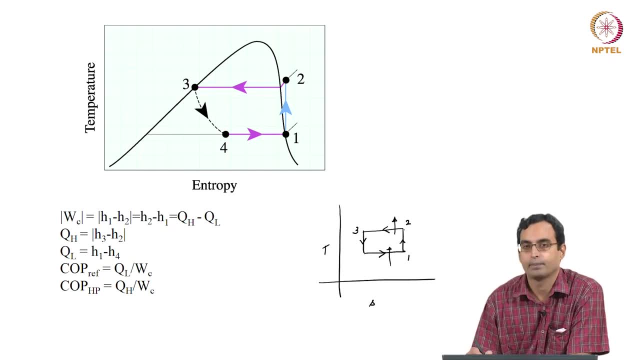 So 2 to 3 is a process of heat rejection. this should be at higher temperature, And 4 to 1 is a process of heat addition to the cycle. it should be at low temperature. So which essentially means that this cycle runs anti-clockwise as compared to our power. 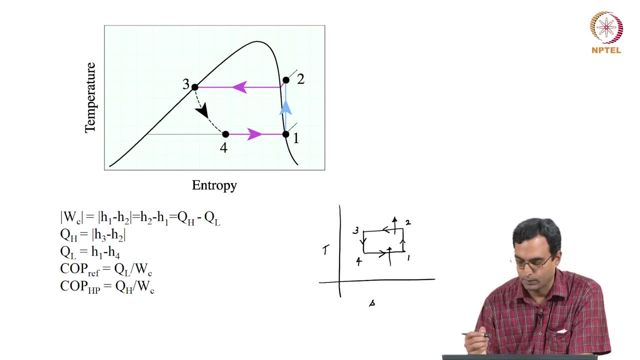 generation cycles which run clockwise on a TS or a PV diagram. So ideally we would like this cycle But, as we discussed earlier, it is hard to have processes 1 to 4, 4 to 1 and 2 to 3 as 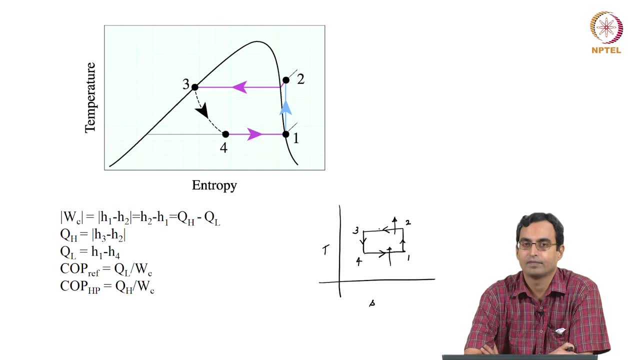 well, So we can do isothermal heat addition and heat rejection when we are using single phase flow. What is easier to do is to do constant pressure heat addition or constant pressure heat rejection, And one of the ways in which we can achieve both a constant pressure and constant temperature. 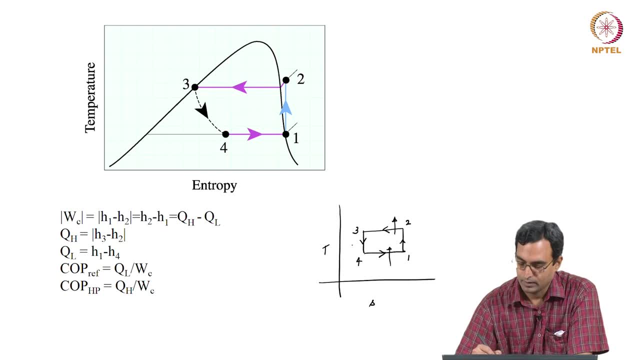 process is to put this into a liquid vapor dome to use two-phase flows. So that is essentially what we do. like in the other cases, We do this with a two-phase mixture. We can, Because then a constant pressure process is the same as a constant temperature process. 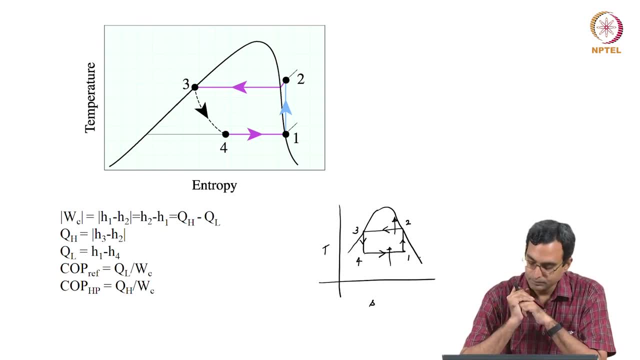 and constant pressure processes are something which we can achieve. So this is a modification which we would first do. instead of using a single phase substance, we could do this in a two-phase mixture and then run what would be a Carnot cycle. But, as we saw in the case of, say, the Rankine cycle, we also have problems here, because 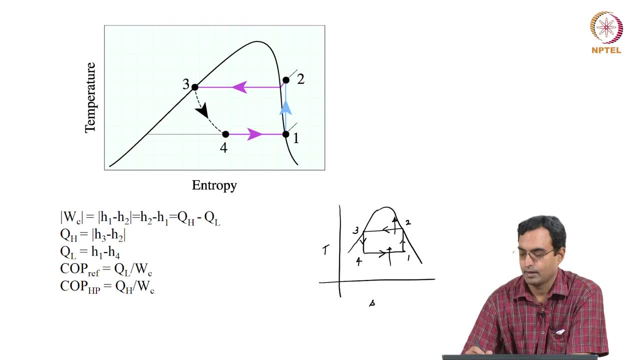 once we have a two-phase mixture. Now we are trying to compress a mixture of liquid and vapor, Because if I want this entire cycle to be in the dome, the dome should pass through these points 2 and 3 or it should be smaller. 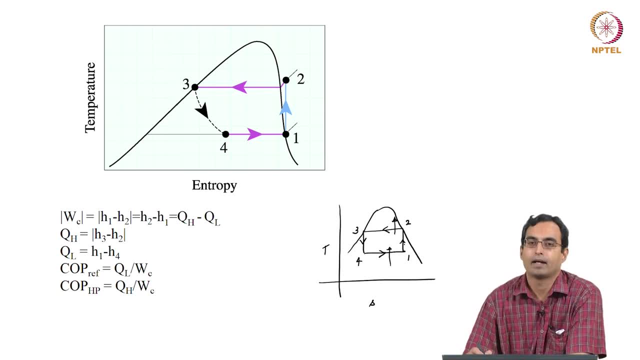 And in that case what I am compressing here- 1 to 2- is compression. ideally it should be isentropic compression, reversible adiabatic compression. But in this process- 1 to 2, I am trying to compress a mixture of liquid and vapor at 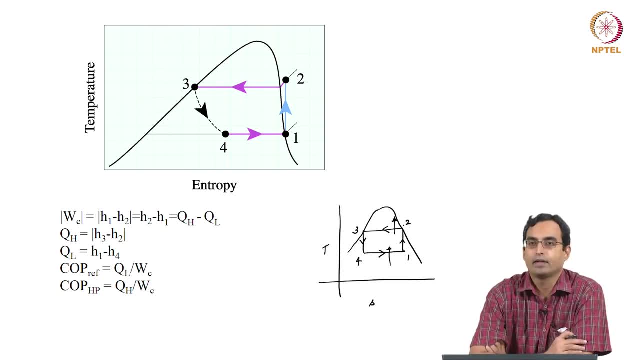 1 and get only vapor at 2.. It is 2.. It is 2.. So it is difficult to find compressors which can deal with two-phase mixtures and do this efficiently and do this without getting damaged. So what we would like to ideally do is to make sure that in the compressor there is 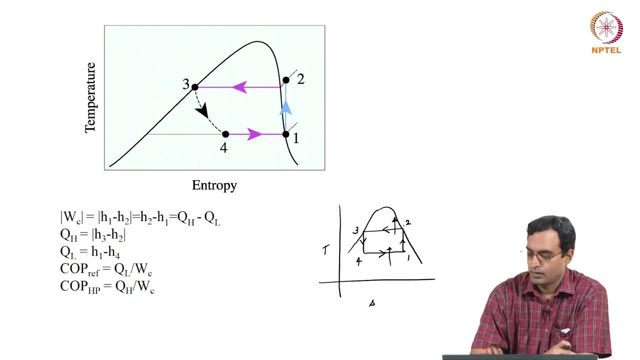 only a single phase. So we cannot. so, which means that we should do all compression either in liquid, which does not help us because in that case the entire cycle is going to be in the liquid, or we can do the compression in the vapor phase. 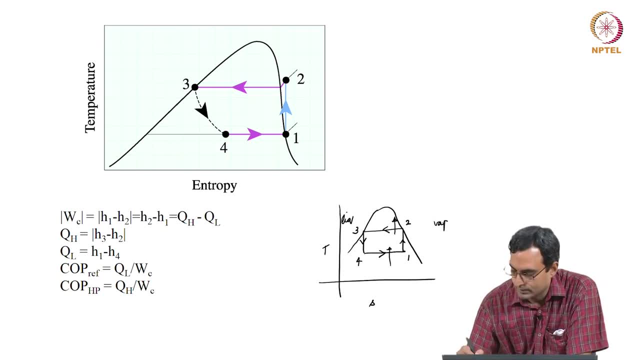 So here we have liquid, Here we have vapor, Here we have a two-phase mixture which we represent as 2 phi. So what we would like to do is to move this compression out of this mixture. So one way we have to do that is to essentially move this point 1 to the saturated vapor line. 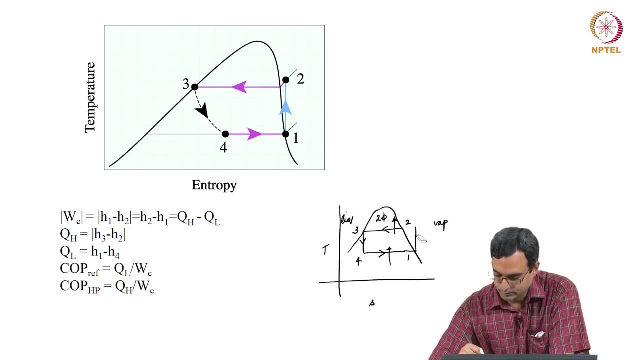 and then compress from here. This will still be isentropic compression, So it will be a straight line compression. So it will still be isentropic compression, So it will be a straight line compression. Then, parallel to the T-axis, we can compress like this: 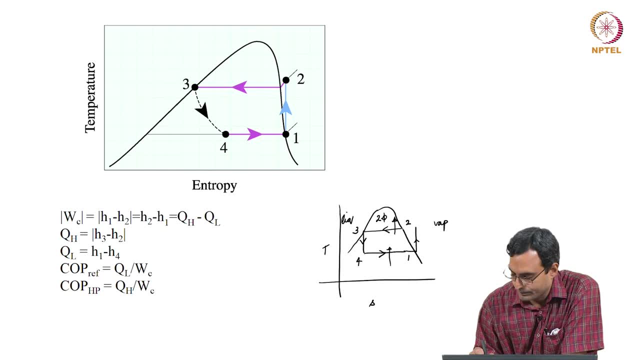 So if we compress up to this temperature 2 to 3, and if we wanted to do this, then what we would see is this portion, the dotted region, would essentially be isothermal compression. The process from 2 to 3 is isothermal but, more importantly, it is constant pressure heat. 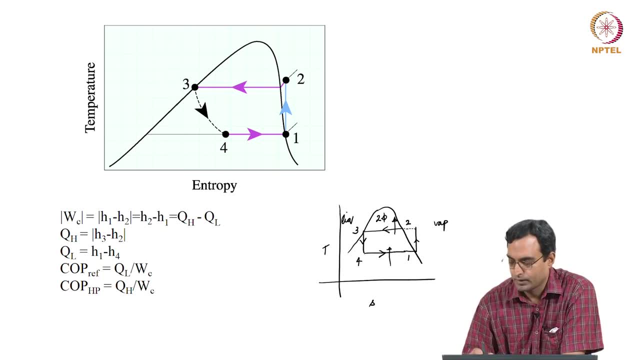 rejection. But this portion, the dotted portion, would be isothermal heat rejection, which is difficult to achieve. So this is not very feasible. So what is feasible is to make the heat rejection process, which is essentially this portion as well as this portion, make those at the same pressure. 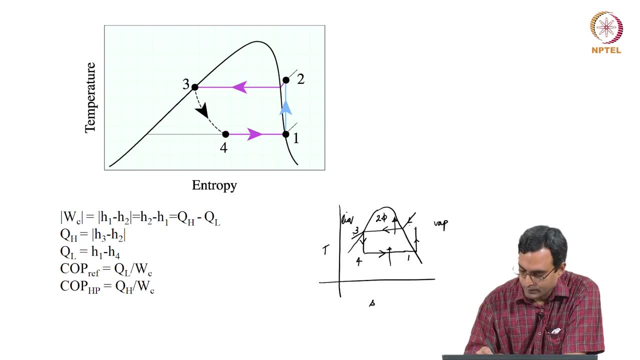 So we can draw this isobar, which is Okay, See Okay. The isobar is essentially this line. that is what an isobar looks like on the TS diagram. So what we are trying to do is make use of that isobar. 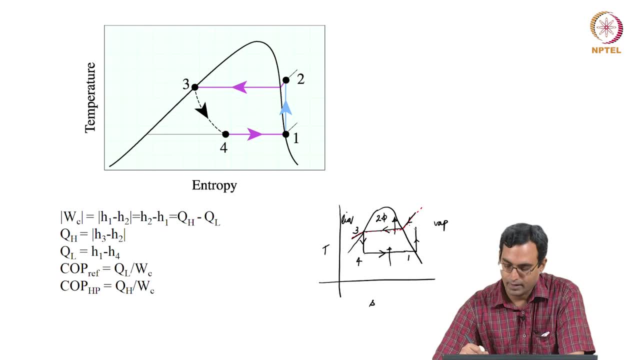 So instead of compressing to the pressure at this point, we compress to the pressure at 3.. So if the isobar at 3 over here passes through this point, so what we see is this: 3, and let me call this point as some, A and this point as some. this point is 2.. 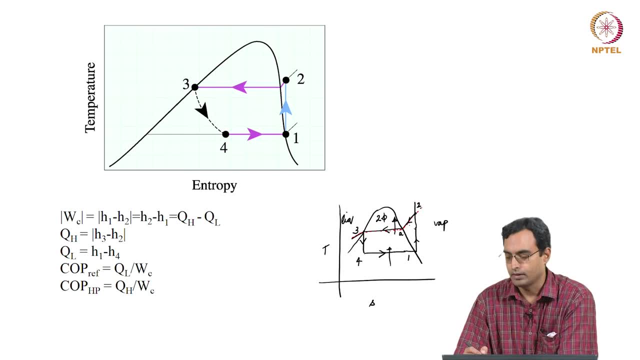 So this pressure at 3, A and 2 is the same. So in order to reach that pressure, what we need to do is we need to compress to a higher temperature in the vapor region. The pressure is still the same at 3 and at A and at 2, because this is an isobar. but 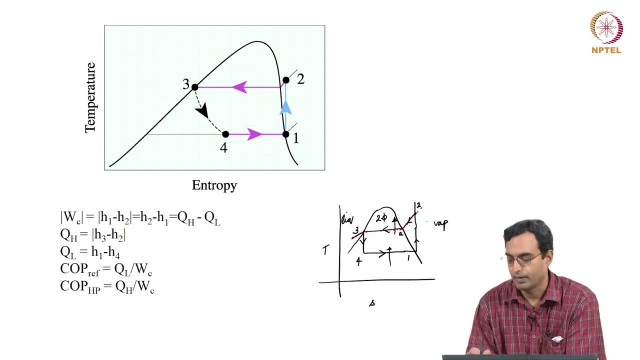 the temperature is different When you are in the vapor region, when you are in the two-phase region and- let us say some point over here- in the liquid region. the pressure is different in the sorry, the pressure is the same, but the temperature is different at different points in this region. 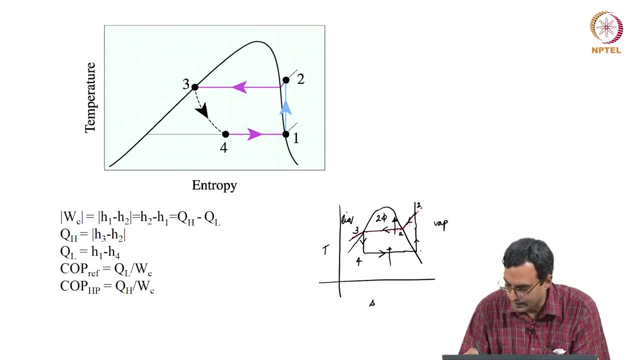 So we are now left with this cycle which starts at saturated vapor, dry saturated vapor at 0.1.. We are compressing to some temperature- T2.. The pressure at 2, A and 3 are the same. Then we can do constant pressure heat rejection in a heat exchanger from 2 to 3.. 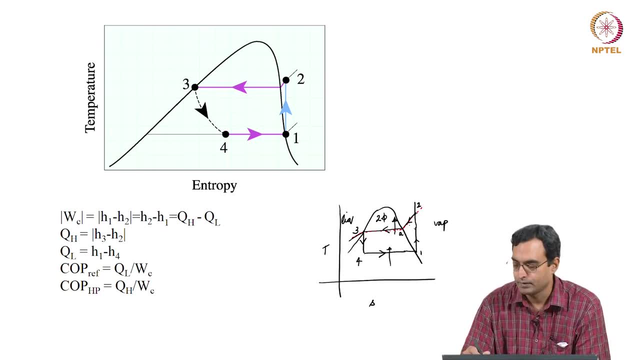 This heat exchanger is a heat exchanger where we have vapor becoming liquid. So the process is happening by condensation. So we call this heat exchanger as a condenser and we are left with liquid at 0.3.. Now 3 to 4 is an expansion process. 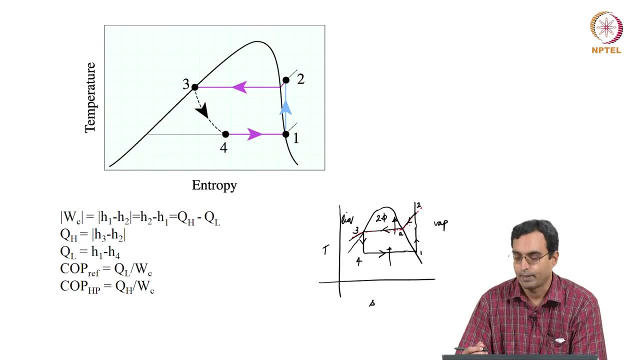 In the Carnot cycle. this would be a reversible adiabatic expansion. So we are left with liquid at 0.3.. Now, 3 to 4 is an expansion process In the Carnot cycle. this would be a reversible adiabatic expansion or isentropic expansion. 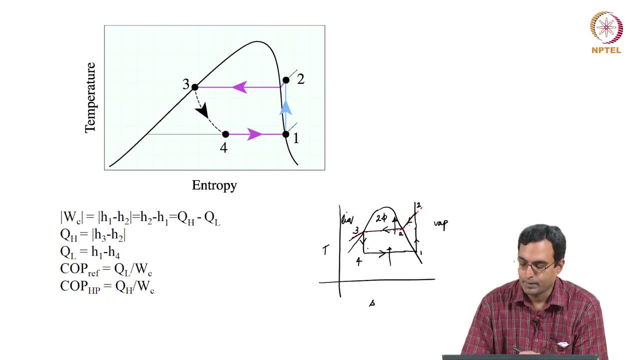 We would ideally do this in a turbine, But we have seen issues with using a turbine in two-phase mixtures earlier. So again, we are starting with liquid at 3.. At 0.4, we are in between the liquid line and the vapor line, which means it is a mixture. 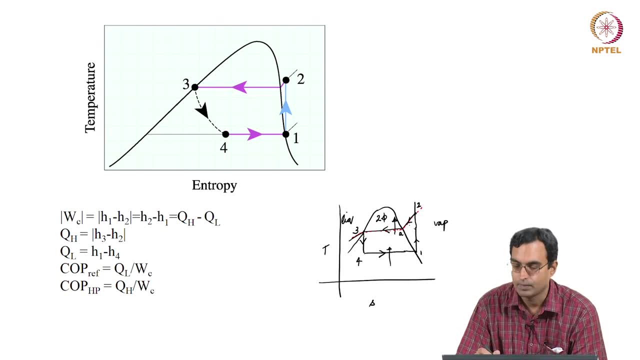 of liquid and vapor. So we are going to have problems with liquid droplets hitting the blades and damaging the blades. That is one potential problem which we would have, But there is also another issue. So we saw that the work in the turbine would be given as the specific work would be essentially. 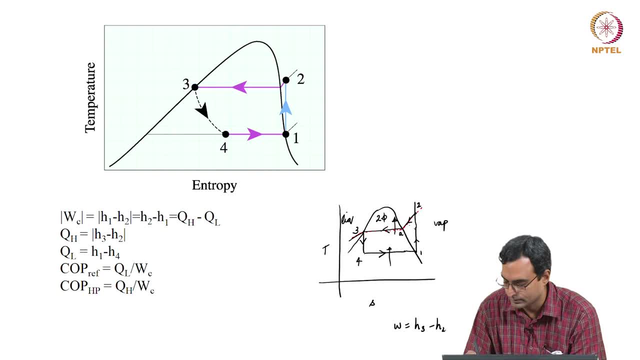 the change in the enthalpy between the inlet and the outlet, Assuming that there is no change in potential and kinetic energy and assuming that this is adiabatic and its steady state. this would be the kind of work we get And we saw that for an isentropic process we can also write this as integral of Vdp. 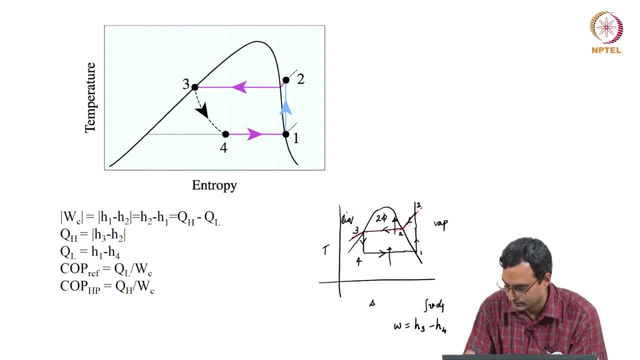 So we are left with liquid at 0.3.. So we are left with liquid at 0.4.. And what we see over here is we are close to the liquid line. So if we are close to the liquid line, then the specific volume is small. 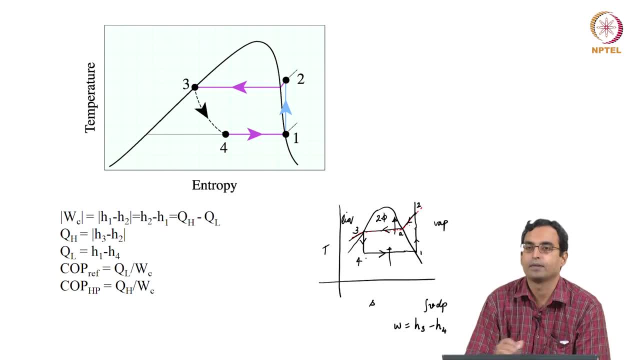 The specific volume of vapors is very high. The specific volume of liquids are small because the density of liquids are large. So even when we are at 0.4, we are closer to the liquid line than to the vapor line, which means that the specific volume will be small. 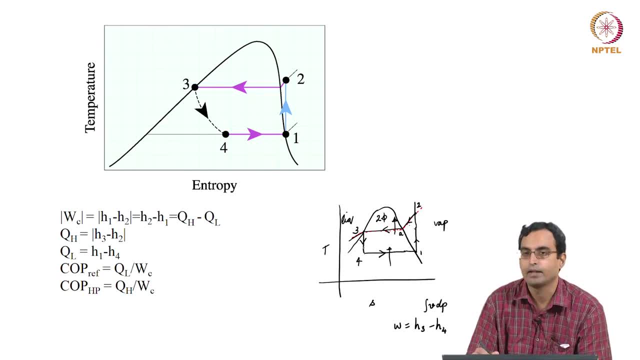 So we are close to the liquid line. So the amount of work we can get by putting this turbine here is fairly small. A turbine is an expensive device. We want to, for example, manufacture a fridge and sell it. So let us say a fridge costs something like, say, 10,000 rupees or something like that. 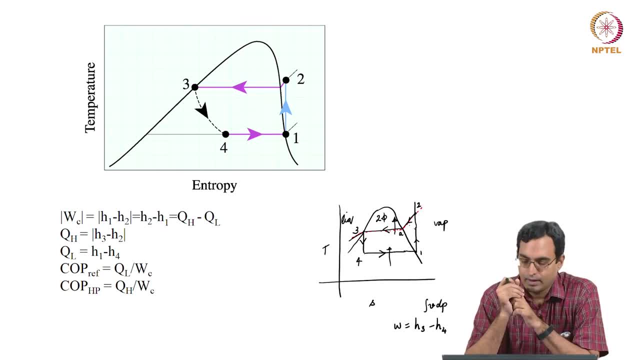 or say 15,000 rupees. If we make a turbine, it would be very expensive, So it would increase the price of the fridge by a large amount and we will not get much work because specific volume is small And we want to make a turbine. 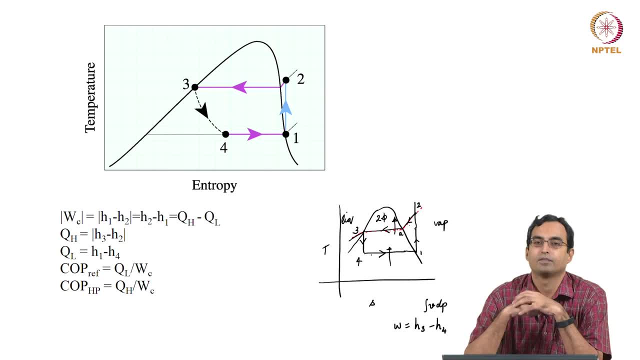 And the turbine would possibly get damaged because it is dealing with two-phase mixtures. So all of these leads us to the conclusion that putting a turbine here, even though it is useful to improve the efficiency of the cycle, it is possibly not going to be very. 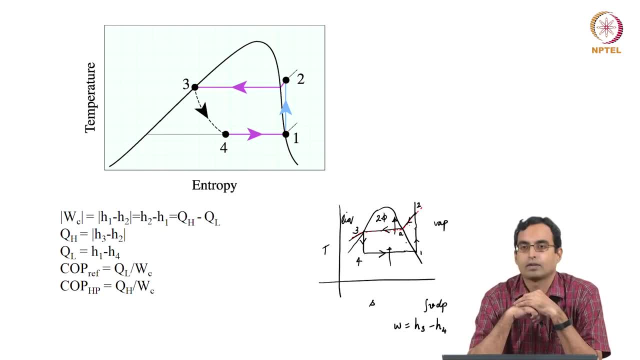 feasible from a cost perspective and from durability of this device. So what we usually do is we remove the turbine and we put a throttling device. a throttling device can be essentially a valve. it can also just be a tube with very small diameter. 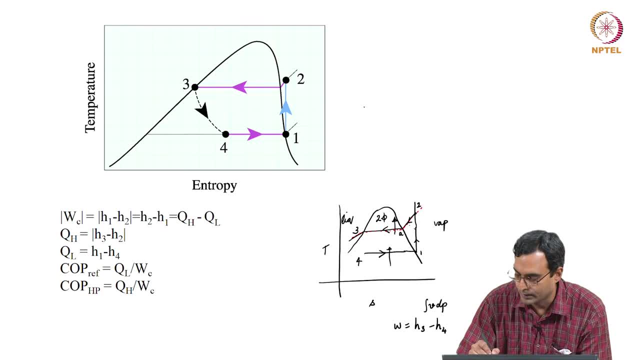 So we put a throttling device. so, for example, if you have liquid coming at point 3 and then you make it pass through a long tube whose diameter is very small, there will be lot of pressure. So this process in this tube because of friction. so typically this tube is extremely long and 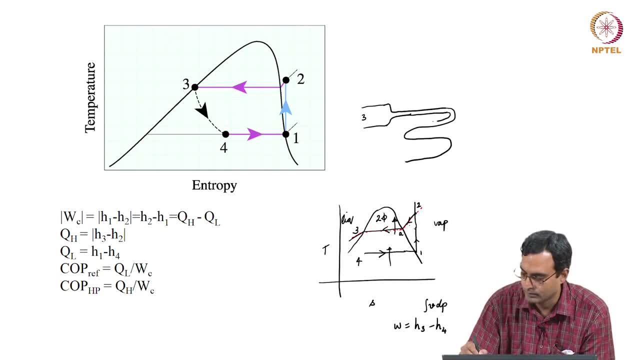 you can coil it around of course. you would possibly have the same diameter. I have not drawn it all that well, but what we see is when this liquid flows in through this tube, it has viscosity, so it has a lot of pressure drop, so the pressure drops in this case. 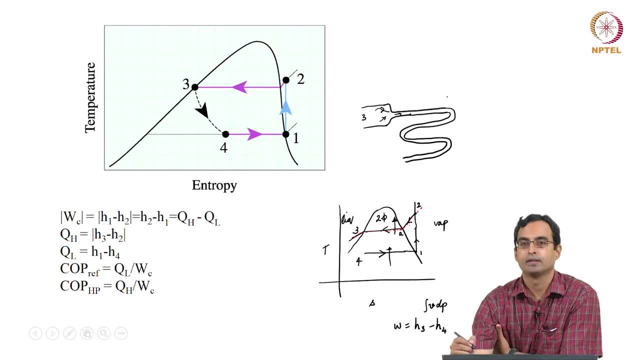 if this flows fast, We can assume that this process happens adiabatically. so it is adiabatic, but the pressure is dropping and in this process, what we see is that the enthalpy remains constant. if we ignore, if we assume this to be steady state and if we ignore changes in potential kinetic energy. 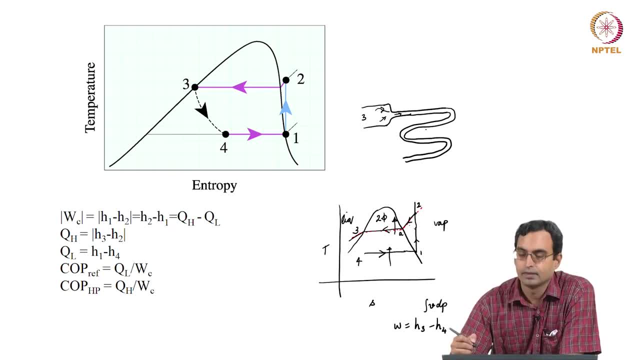 then the enthalpy remains constant and the pressure drops. And for non-ideal gas substances, if you choose the range of initial temperatures correctly, what you would have is usually a temperature drop. Of course, actual case of whether the temperature will drop or increase depends on the Joule-Thompson. 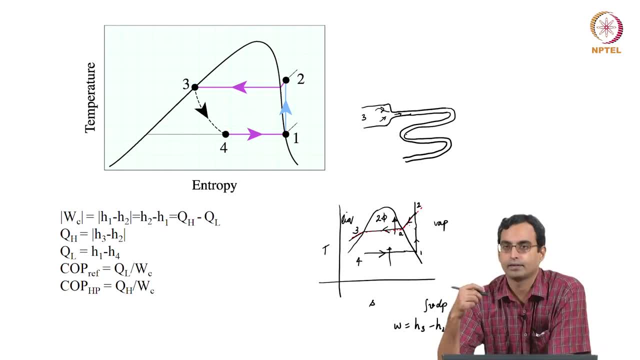 coefficient, but we are in. if you are looking at a gas, it could either increase or reduce In the case of these kind of mixtures which we have here. in the case of liquids of the kind we have here, in this condition the temperature would drop as the pressure drops. 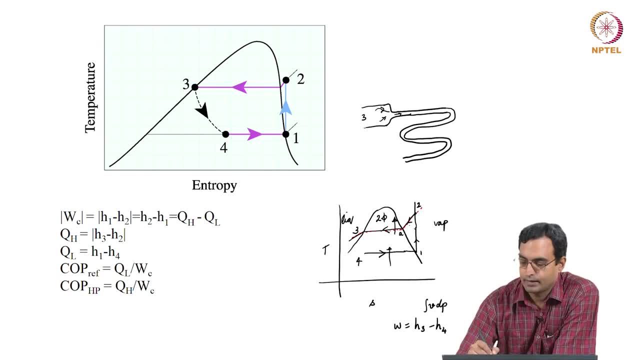 So what we see is: at 3,, the temperature is T3.. At the exit, it is T3.. Okay, At the exit of this, at 4,, the temperature drops from T3 to T4. This is an irreversible process because there is friction, which means that the entropy increases. 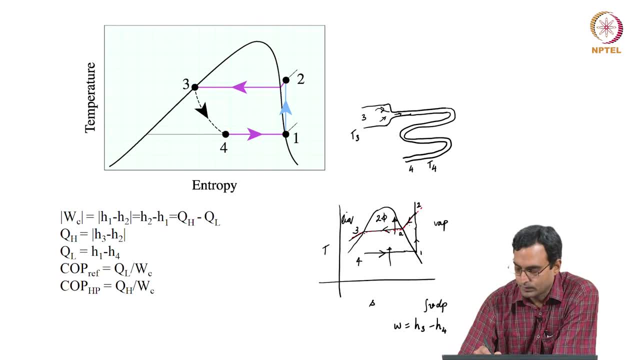 So the entropy increases and the temperature drops. So point 4, the temperature at 4 should be lower, the entropy at 4 should be higher. So this is the entropy at 3, entropy at 4 should be higher, and this is now an irreversible. 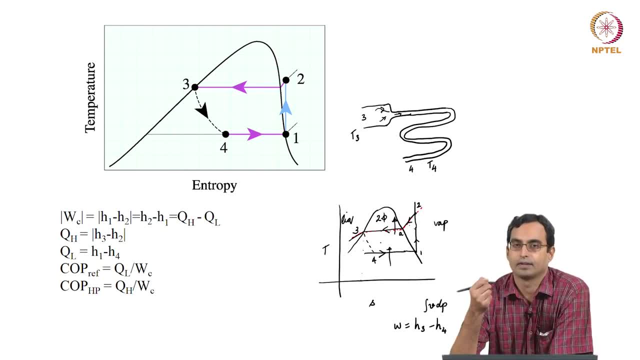 process. So we do not know what this shape of this process is. So, but we are left with now a cycle of this form. So we started with the Carnot cycle. We can modify that into the reverse Rankine cycle by doing this kind of compression here. 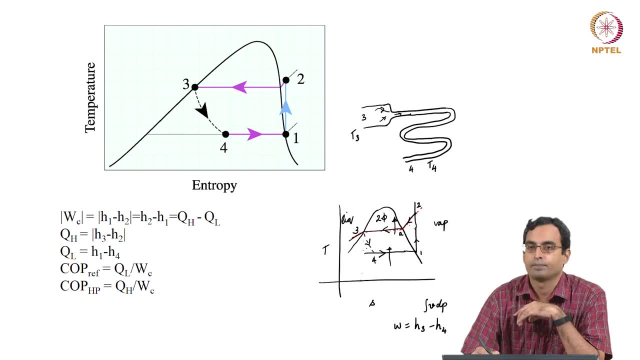 in the vapor region and having a turbine here, But then that is not very useful either, because the turbine is expensive and it has problems. So what we have now done is we have changed it into an isenthalpic process which is called the Carnot cycle. 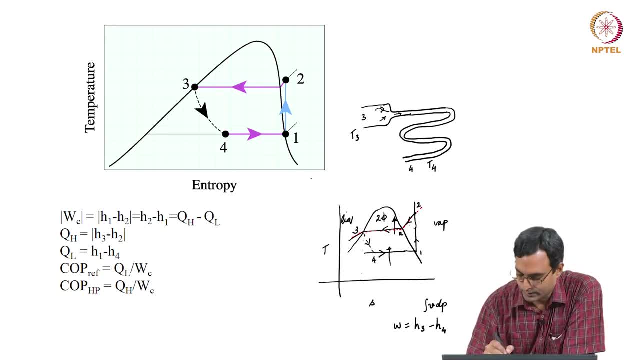 Okay, So it is irreversible. and we are now left with the vapor compression refrigeration system, which is called VCRS in short, which gives us this cycle. So the same cycle is drawn up. Okay, It is drawn over here. So we have 1 to 2, which is isentropic compression, 2 to 3, which is constant pressure, heat rejection. 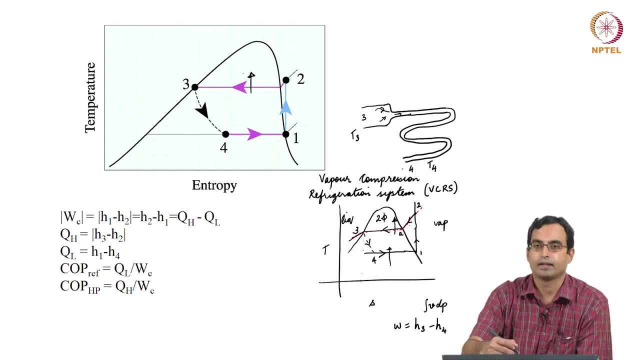 out of this cycle, which is usually heat rejected to the atmosphere. 3 to 4,, which is a throttling process which is adiabatic and irreversible. 4 to 1,, which is constant pressure as well as constant temperature. heat absorption, where we are taking heat from the substance. 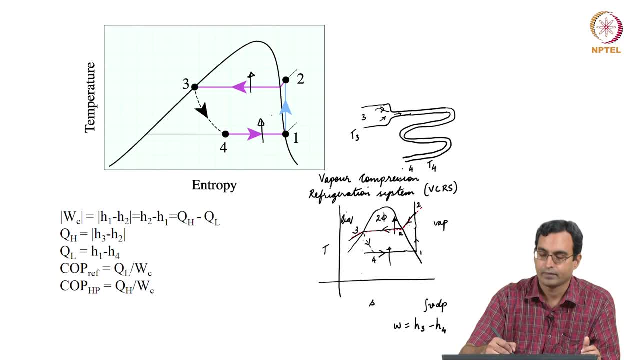 which we want to cool And taking it into the cycle, And then 1 to 2 once again is reversible adiabatic compression. So this is essentially the VCRS cycle which we use instead of the Carnot cycle. So we can look at what are the things which we are doing in this cycle. 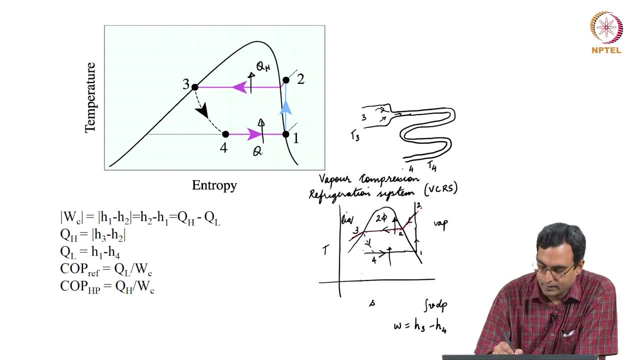 So we have heat rejection here. QH. We have heat absorption into the cycle, which is QL, which is usually what we are interested in. if we are running this as a refrigerator, Okay, If we are running this as a heat pump, we would be interested in this. QH. 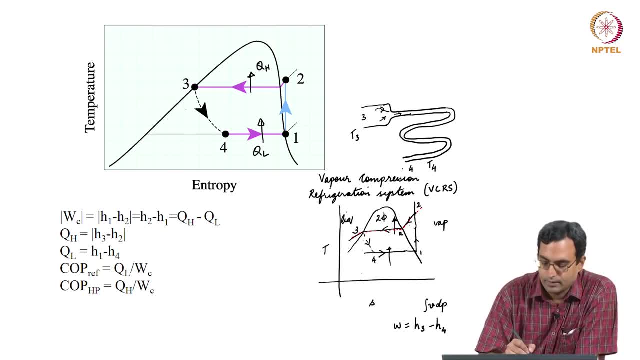 This 3 to 4 is a throttling process. There is no heat transfer in this throttling process. We also do not have work done because there are no moving paths, There is no shaft. There is no change in the cross section of the. there is no change, not in the cross. 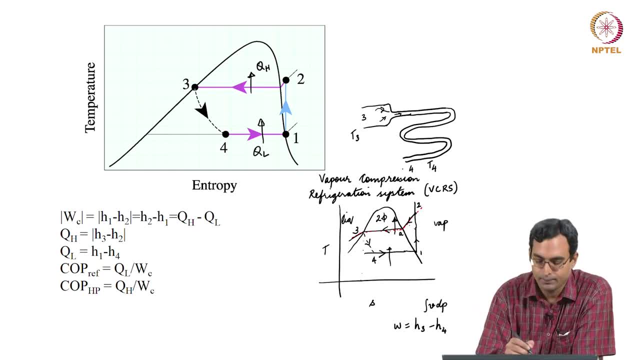 section. there is no change in the volume of the device in which it happens. so we do not have heat transfer here, We do not have work interaction here. Over here we are doing work on the system, So this would be compressor work, which would be negative for this cycle. 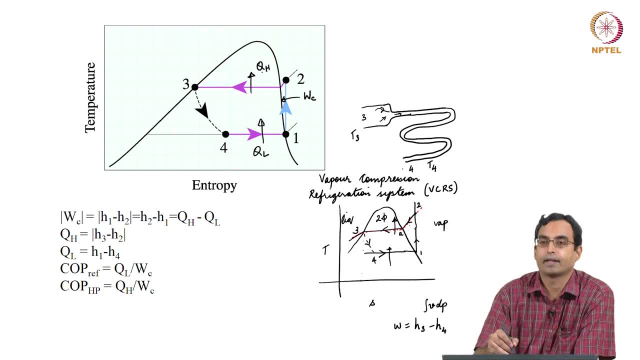 QL is positive for the cycle heat coming in. QH is negative for the cycle. it is heat going out And here we do not have heat or work transfers. So if you want to find out the amount of heat coming in over here, 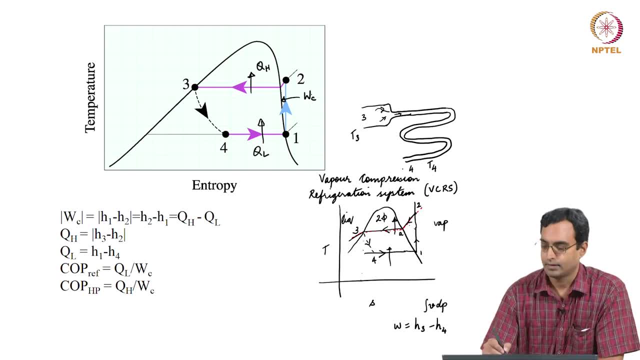 Sorry, The amount of work coming in over here. This is isentropic. There is no heat interaction here. What we have been typically doing is drawing this as some kind of a system of this kind. This is WC. This is QH. 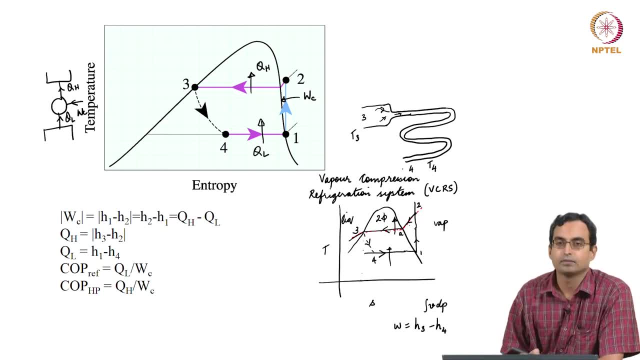 This is QL, So from the first law this is running as a refrigerator. Okay, We have been usually maybe putting the other kind of arrow- I do not know, maybe anti-clockwise, to show that this cycle is anti-clockwise here. maybe. 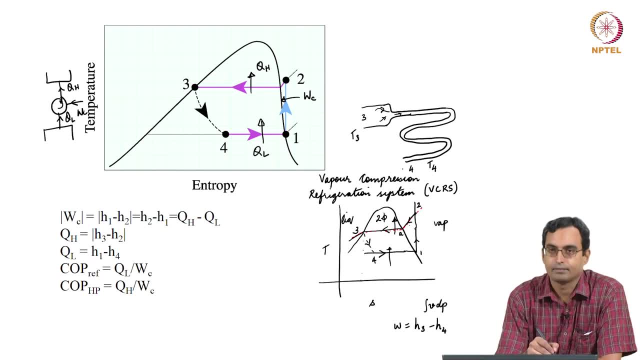 So this is positive, this is negative, this is negative. That is one of the things. And from the first law for a cycle, we have sigma Q equal to sigma W, which says that WC is equal to QH plus QL. 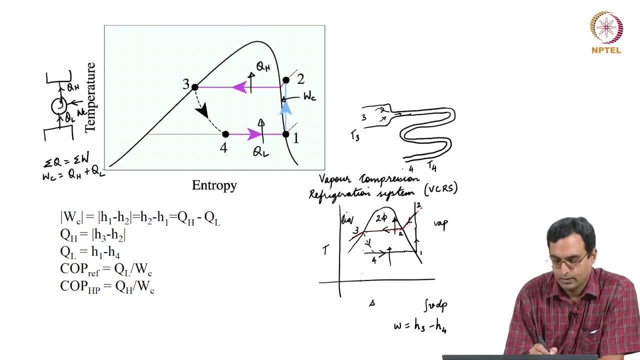 This is negative. this is negative, this is positive. So I would have a negative value here, a negative value here and a positive value here, knowing that these two are negative and this is positive, And what I can do is take mod of this and to find out the positive value, which is essentially. 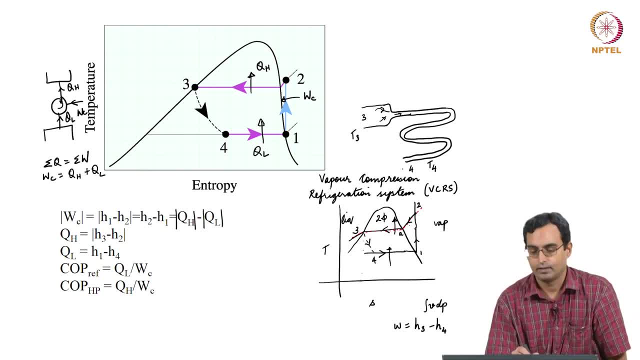 the positive value of QH, the magnitudes, difference in the magnitudes, Because what I know is, if I take only the magnitudes, QL is going here, WC is going here. both these should be added up in magnitude to give me QH. 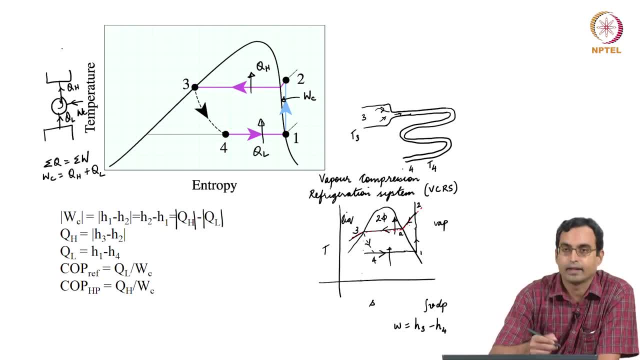 So this is like these two adding up and giving this, because arrows are like that. So that is essentially what I should get. So if I was to write the first law for the compressor, so if I was to look at only the compressor, so the general form of the first law, the compressor, can be treated as a control. 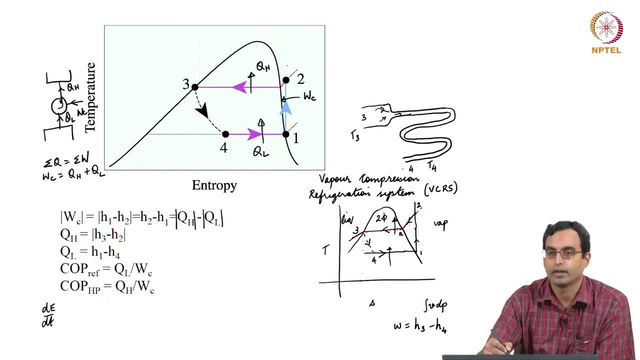 volume where there is some mass, coming in at 1, going out at 2.. So the first law for the compressor would give me this: there is only one inlet and one outlet. I do not need a sigma here. This is the first law. 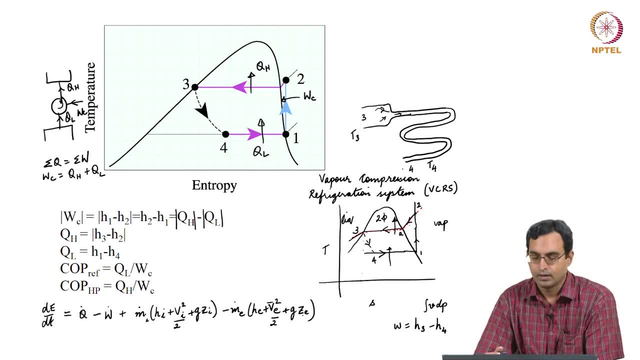 Okay, Thank you. Thank you Now. in addition, we have conservation of mass, which is dm by dt is m dot i minus m dot e. If it is at steady state, this is 0 and m dot i is equal to m dot e, and I can call these: 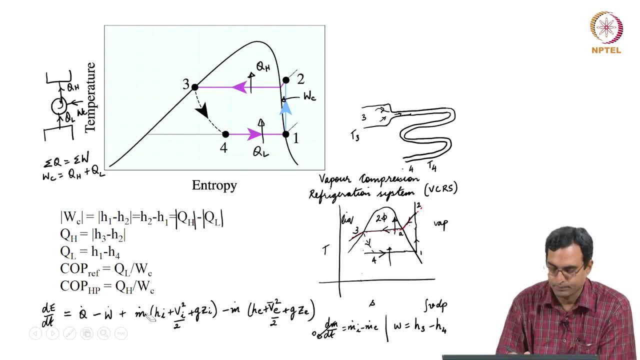 as some m dot, so I can remove the subscripts If it is steady state. this is 0.. For the compressor we expect this to be isentropic, So it is adiabatic and reversible. this is 0. 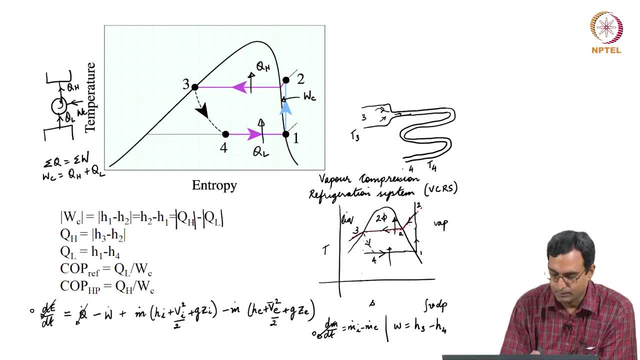 So I can divide this w dot by m dot and call this as some small w. Changes in potential and kinetic energy are usually small, so these are 0.. So what I see is w dot is equal to m dot into inlet enthalpy minus exit enthalpy. 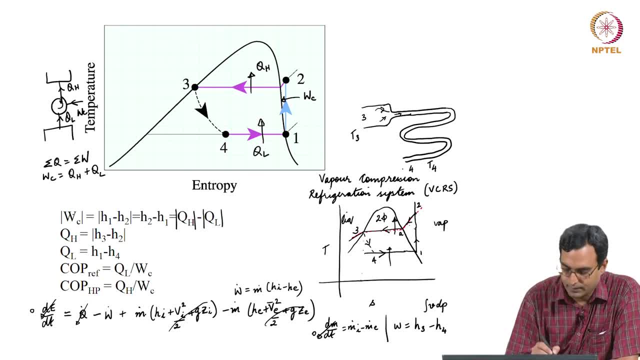 So if I was to write it in terms of capital W, I need an m dot over here. or if I was to write it in terms of small w, I see this is inlet enthalpy minus exit enthalpy for this compressor From the first law. this should also be equal to from the first law for a cyclic process. 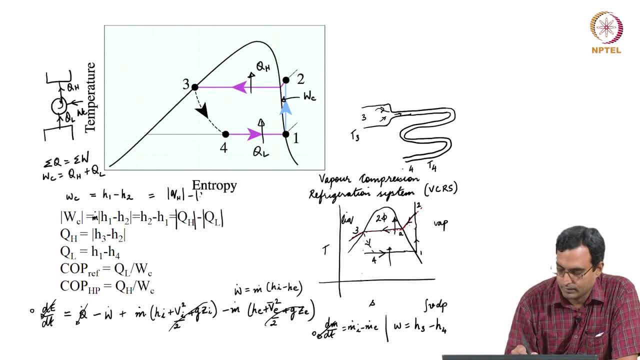 this should also be equal to Qh minus Ql in terms of magnitudes, because Ql is anyway positive. So mod sign here anyway. Now, in a similar fashion, we have found out how much would be the heat transferred. So in the case of, say, 4 to 1, it is a steady process- this is 0.. 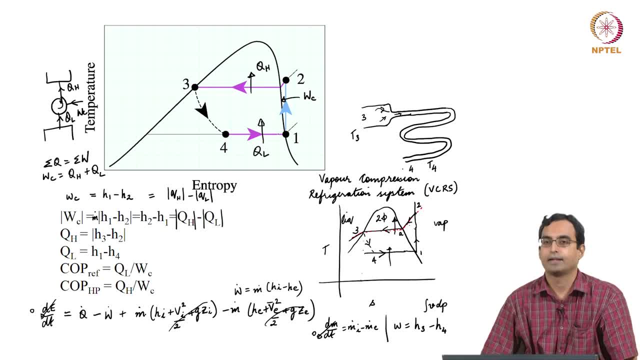 There is no work done, because in 4 to 1, 4 to 1 happens in a heat exchanger There is only flow work, which is already taken into account in enthalpy. There is no displacement work, there is no shaft work, no electrical magnetic work and 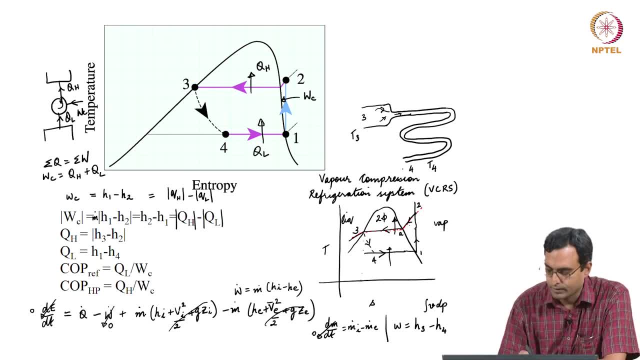 so on. So for the heat exchanger this is 0. Changes in potential energy and kinetic energy are small. it is a steady process. So Q would be m dot into enthalpy at the exit minus enthalpy at the inlet. 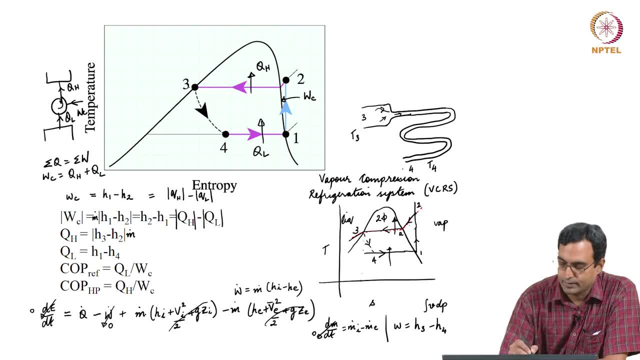 So this is m dot into enthalpy. In this case it is enthalpy at the exit minus enthalpy at inlet. In this case it is enthalpy at exit is 1, inlet is this: this would be m dot into this. 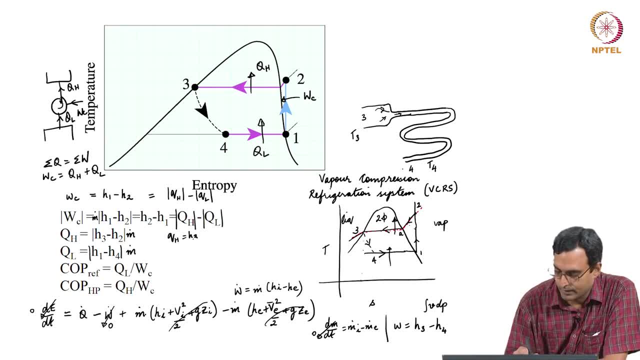 or small. Qh would be h3 minus h2 and small Ql, which is specific heat. So this is m dot, So this is m dot. So the heat transferred would be this. And COP is defined as what we want for a refrigerator. what we want is the amount of 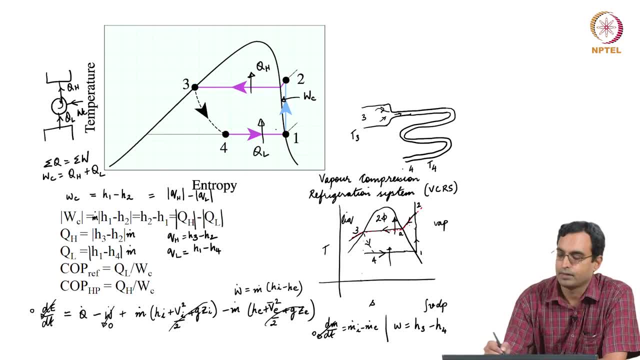 heat we can remove from here, which is Ql, And what we need to give is work in order to run this refrigerator. So for refrigerator the COP would be Ql by Wc, And if it was a heat pump, what we are interested in is how much heat we can get from here to. 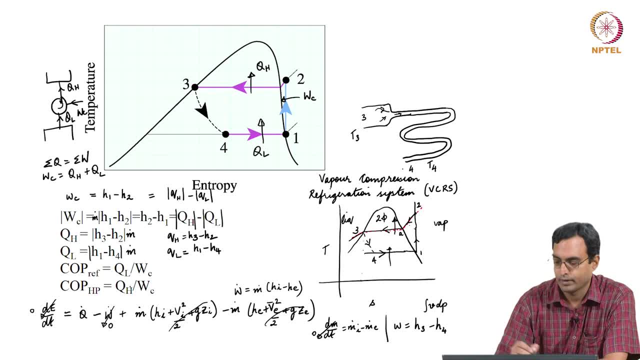 heat a room. So we would be interested in Qh And what we need to give is Wc. So that is essentially what we see, And for the throttling process: we can also write what we get For the throttling process. it is still a steady process.